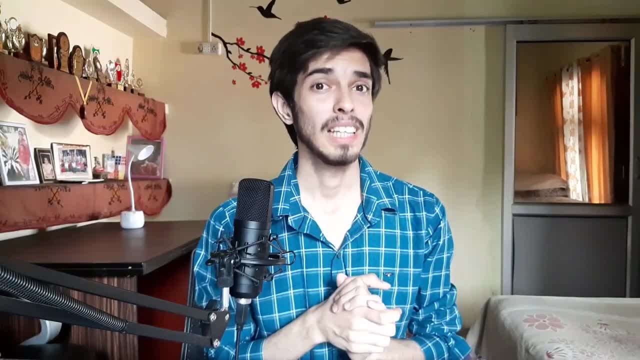 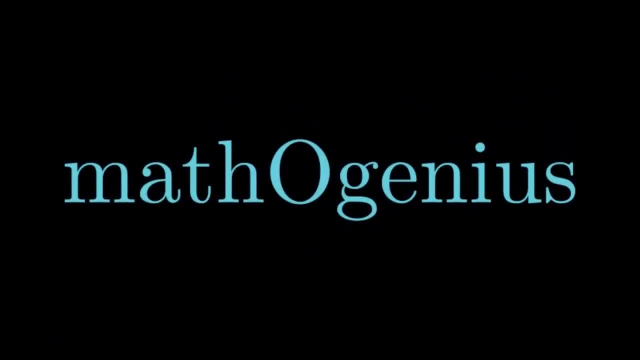 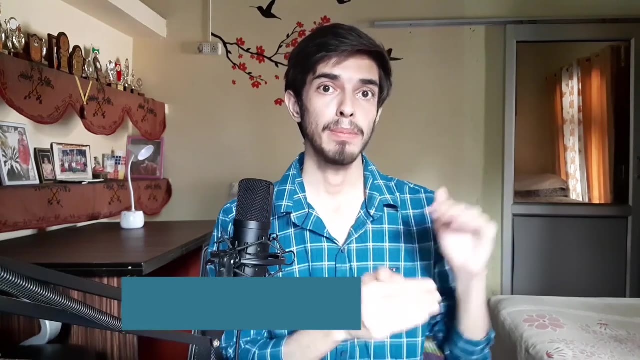 from the date given to him, And in this video we will learn that. so let's begin. Intro. So hello geniuses, Welcome to this another video in Matho Genius Mental Math series. Now, before learning the main method, let us learn its simpler version so that you can get a feel. 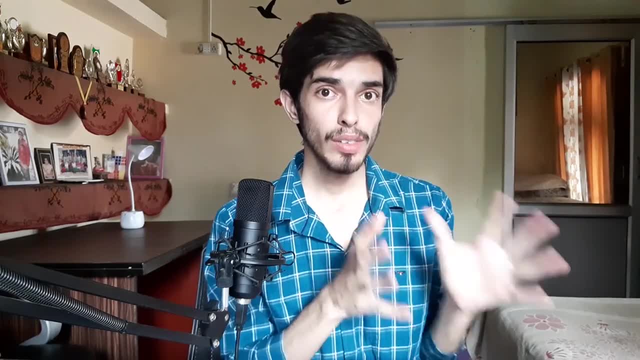 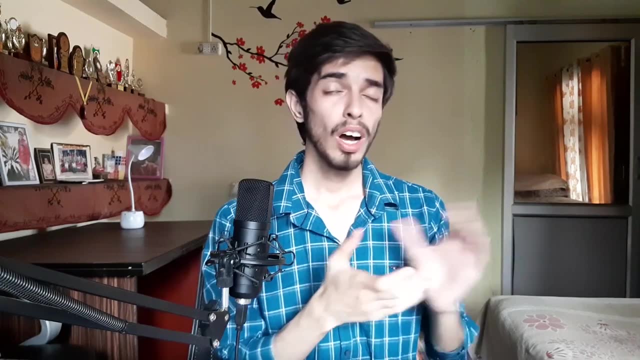 of how this trick works. So in this simpler version, we will figure out the day of January 1st of any year in the 21st century. So how we are gonna do it. First thing is that we are going to learn the day of January 1st of any year in the 21st century. So how we are gonna do it. First thing is that we 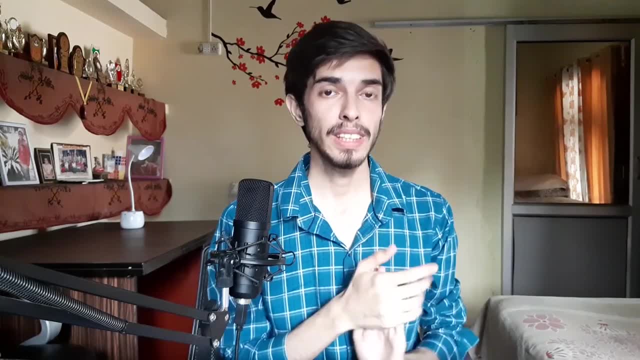 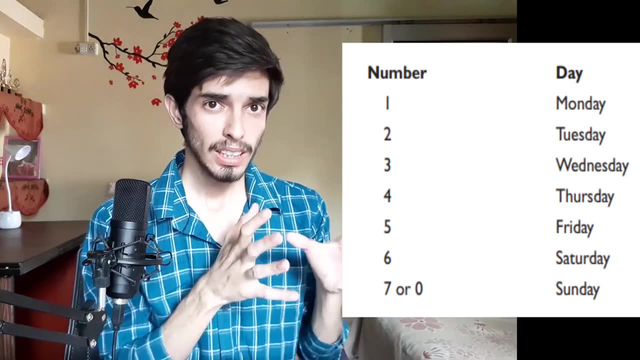 need to associate a number with the days of the weeks, like this. So it's pretty simple. like 1 is for Monday, 2 is for Tuesday, and so on. The only thing you need to take care in here is that. 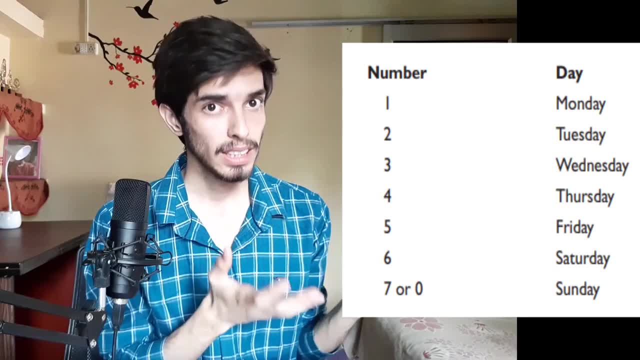 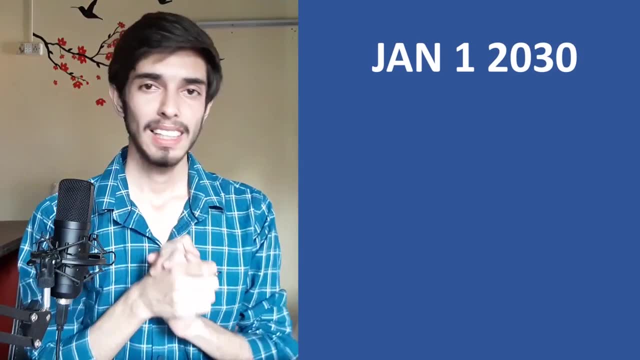 7 and 0 are both associated with Sunday. Now let us calculate the day of the week of January 1, 2030.. So the trick is really simple. Take the last two digits of the year, See in here we have 30.. Now 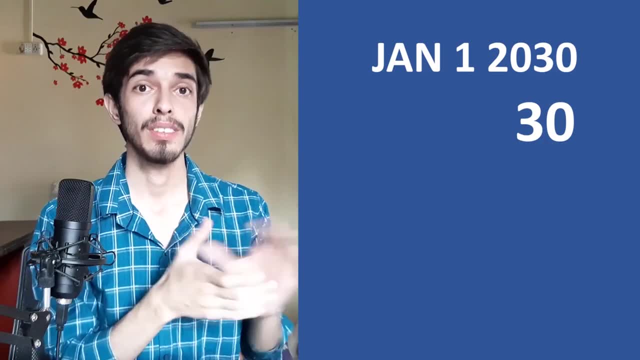 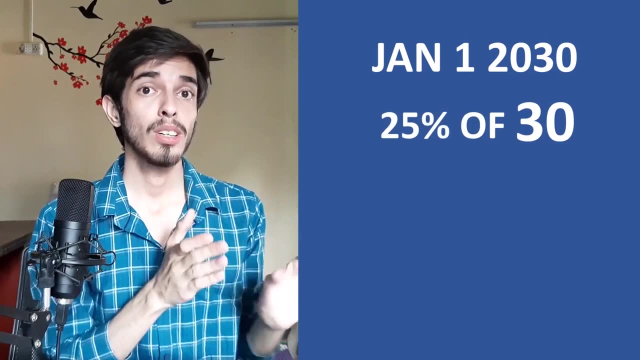 consider it to be your bill at a restaurant. So let's say we have a $30 bill. Now we need to add 25% TIP to it. Okay, so first we need to calculate 25% of 30, which is really simple, See. 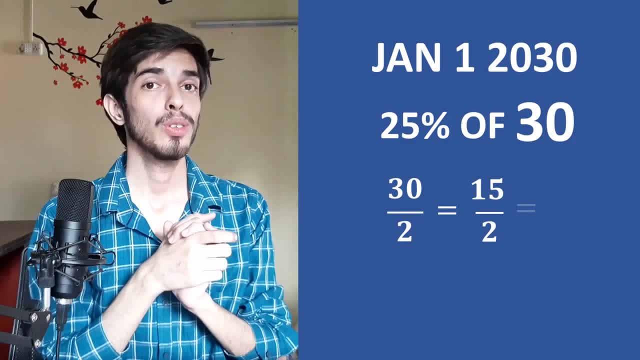 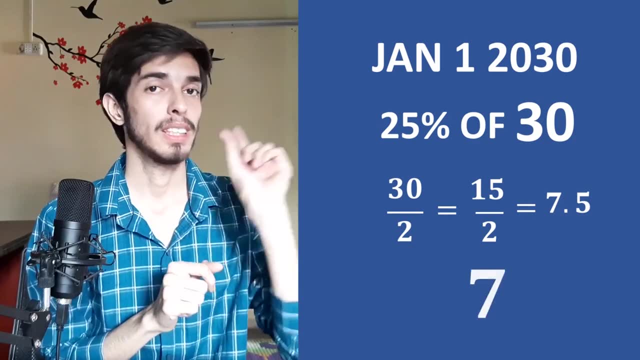 1 half of 30 is 15, which is 50%, and 1 half of 15 is 7.5. So we need to keep the change, don't give the change. So we have 7$ TIP. so keeping that simply means that you don't need to include a point. 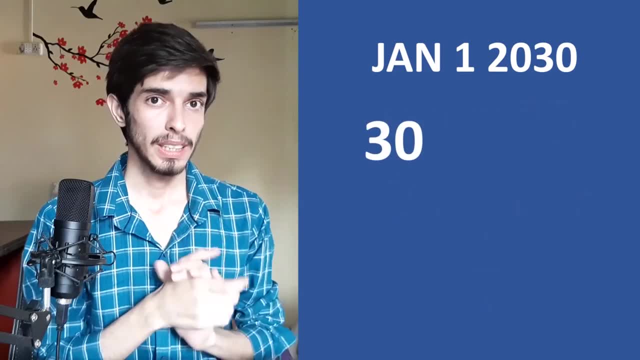 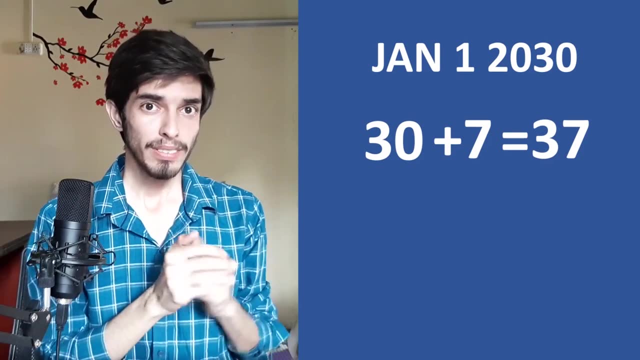 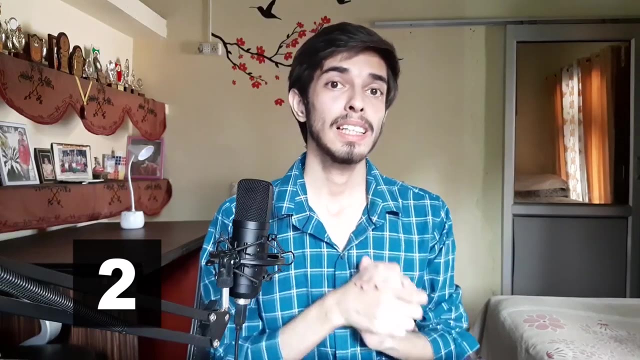 or anything. okay, so seven dollar tip. so our bill is basically 30 plus 7, which is 37 dollars. now we have seven days in a week, so divide it by seven, so seven fives are 35 and we have a remainder two. now this two is basically the code which is associated with the name of the week. 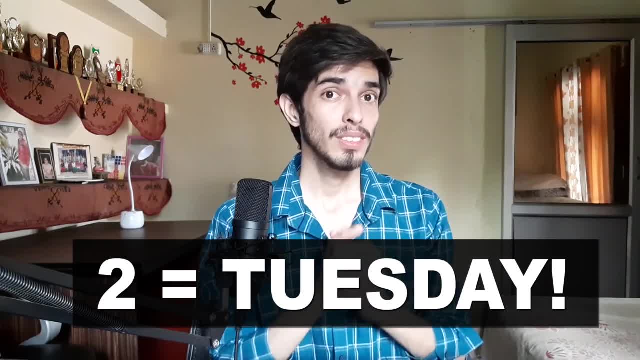 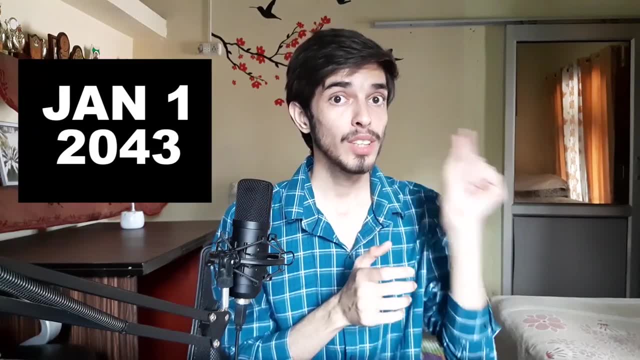 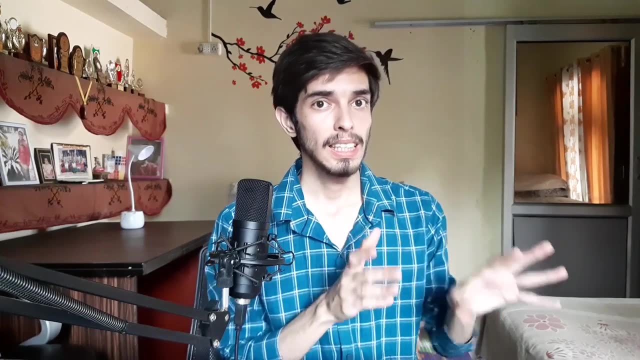 so two was for tuesday, so at january 1- 2030 it will be a tuesday. now, as an exercise, try to calculate the day of the week of january 1- 2043 now in this simpler version. there is just one exception: whenever there is a leap year, you need to subtract 1 dollar from your tip. let's take an. 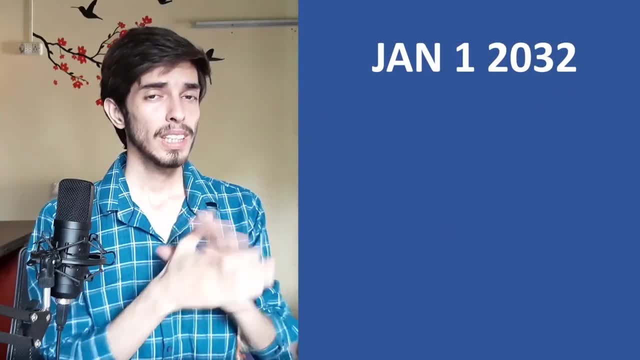 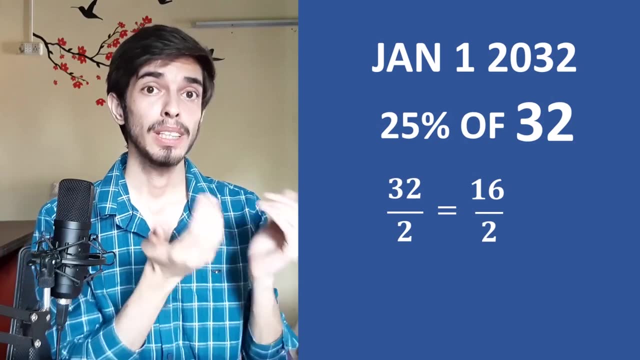 example january 1 of 2032. so first let's calculate 25 percent of 32. so 32 divided by 2, 16, 16 divided by 2, 8. now this is a leap year, so subtract one dollar from it, so we have. 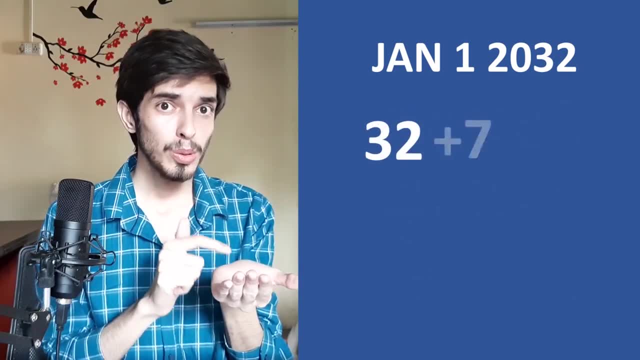 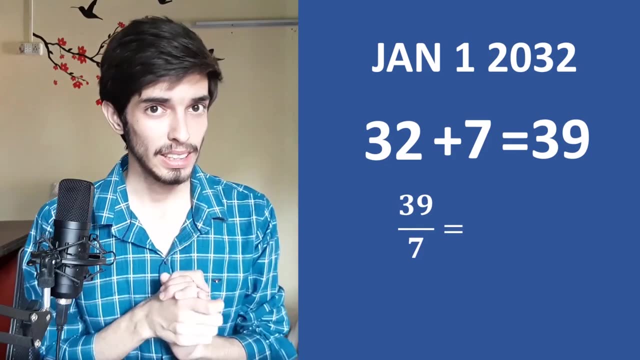 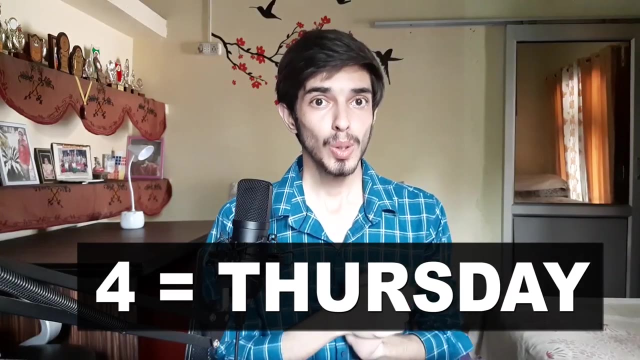 have 7. now our bill is basically 32 plus 7, which is 39 dollars now, simply we need to divide it by 7, because there are 7 days in a week. so 7- 5s are 35, so we have 4 and 4 was for thursday, so at 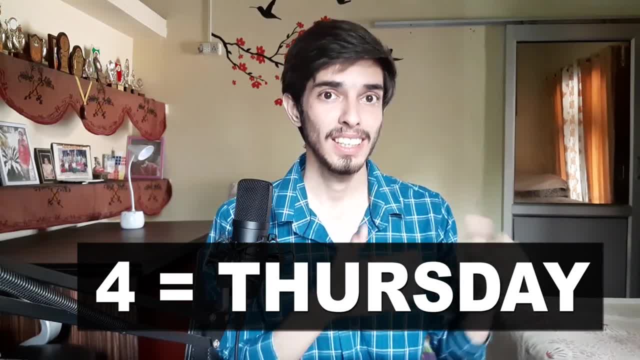 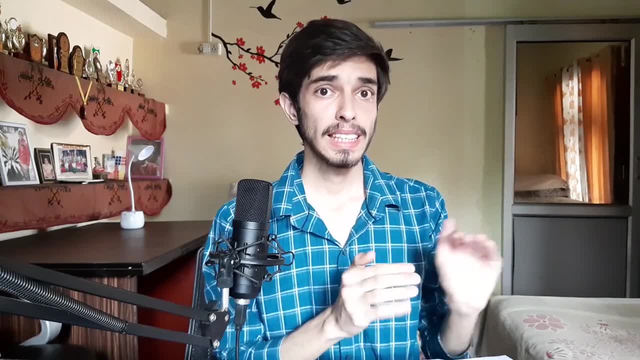 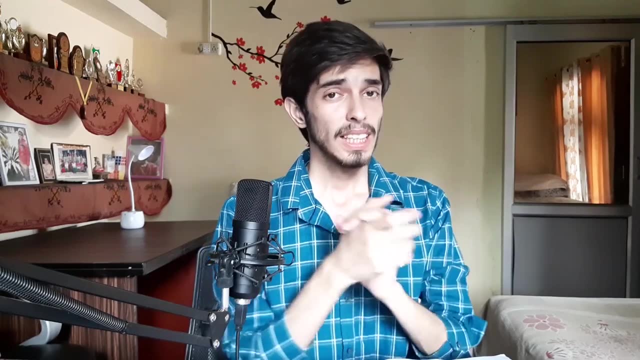 january 1, 2032, there will be a thursday. so see how cool is this? just from the date, you are calculating the day in seconds. now practice with some of the dates and if you are comfortable with this simpler version, then move on to the next advanced version of this trick. now, this advanced version of 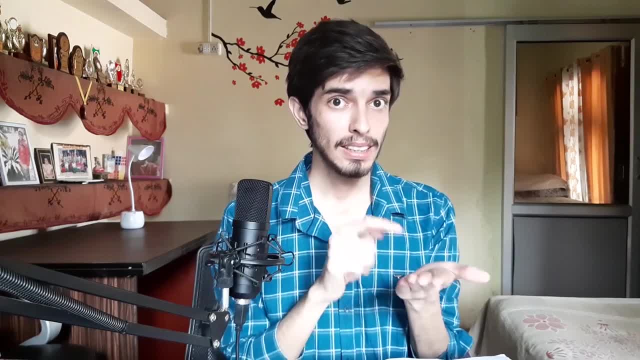 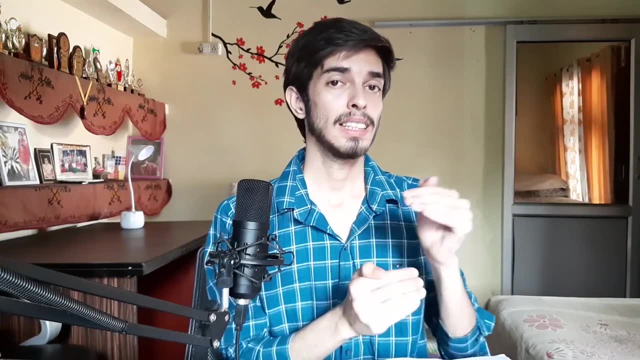 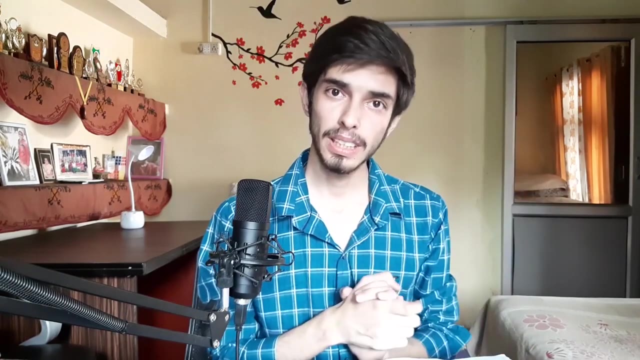 this trick works by assigning codes to days, months and years, and the date itself is also a code. so the only thing difficult in this trick is the month codes, because you need to remember 12 numbers associated with 12 months. okay, you need to remember 12 numbers associated with 12 months, okay. 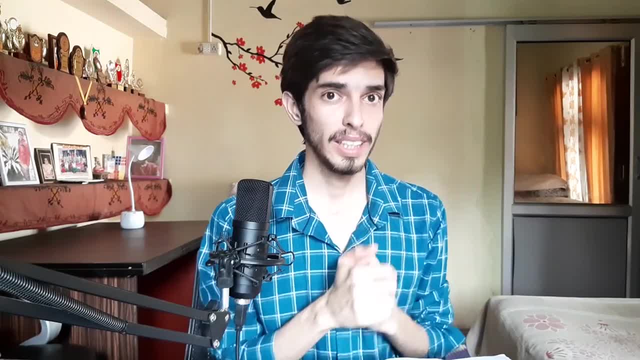 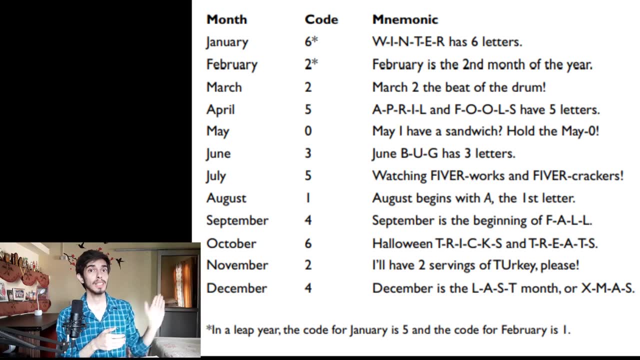 you need to remember 12 numbers associated with 12 months. okay, but there are some mnemonics for it, given by sir arthur benjamin. so the first thing that you need to do is look at this table. in this table there is this month and there is this code number associated with it, and with that there is a mnemonic given to it. read it and try to associate these numbers with these months and remember that for leap years, the code of january is 5 and the code of february is 1. now you can just pause this video and try to memorize this. 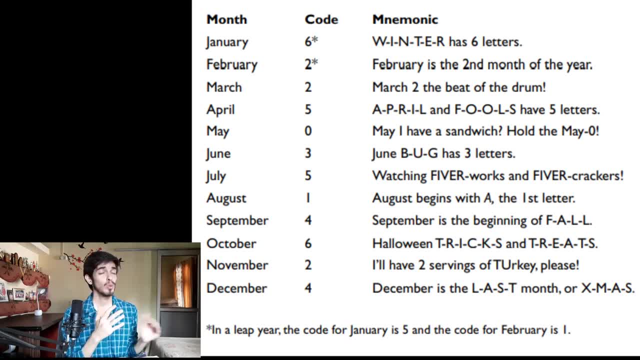 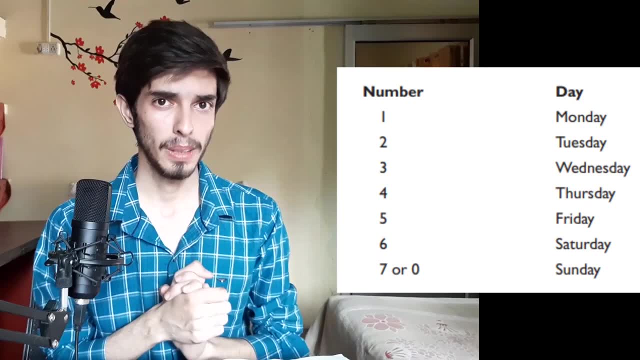 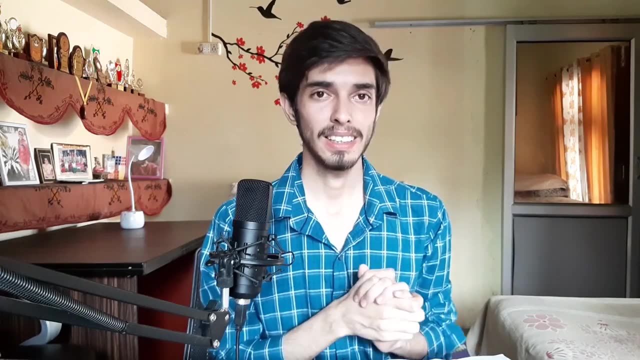 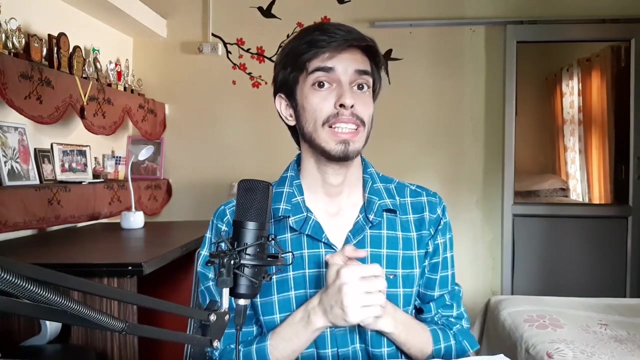 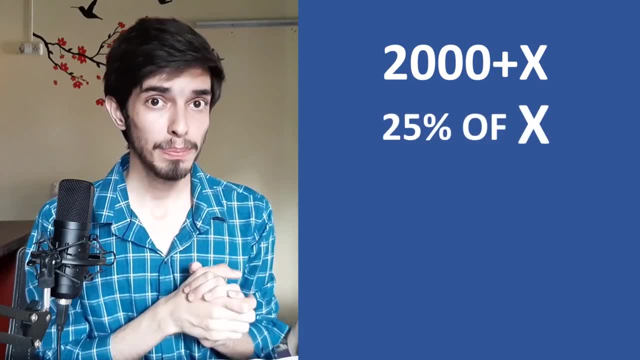 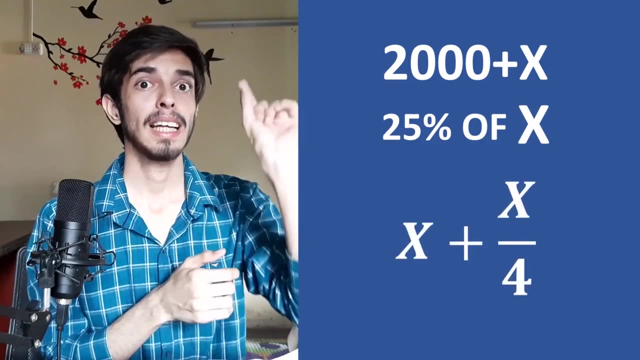 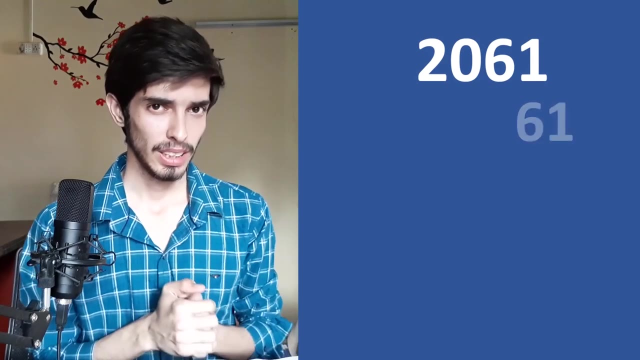 simple, if you have done that before, calculate the 25 tip of this x thing. this x thing is basically the last two digits. so what you need to do is this x plus x by 4. so let us do one exercise: calculate the year code of 2061. do it yourself first. so half of 61 is 30.5 and half of 30.5. 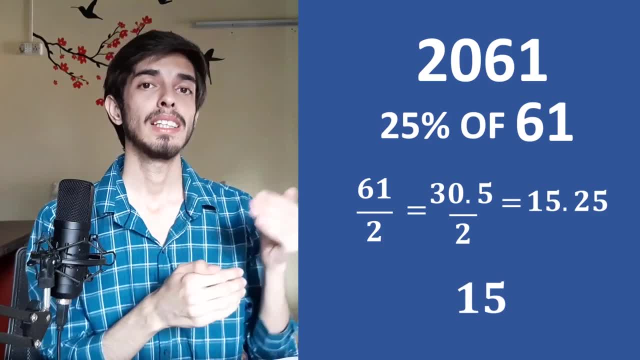 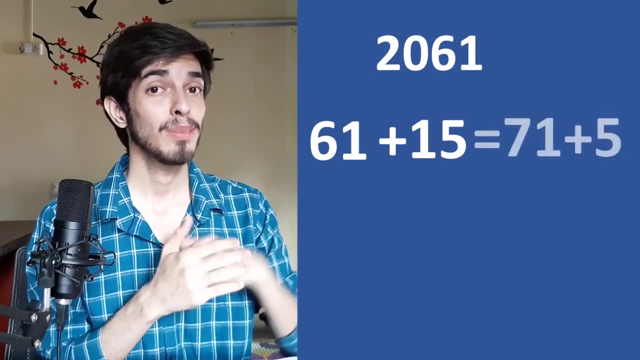 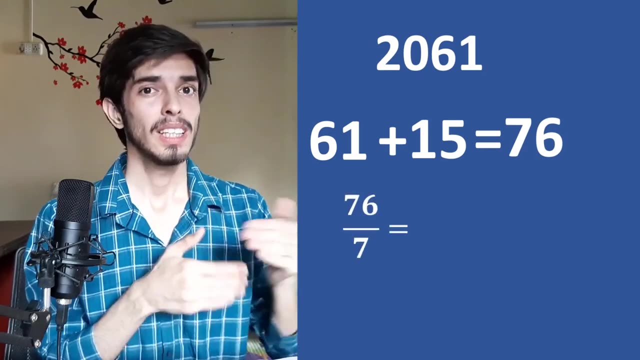 is 15.25, so our tip is 15 dollars. now add this to those two digits, so 61 plus 15. so left to right method: 71 plus 5, 76. now we have 76. now divide it by 7. dividing by 7 is really important, so 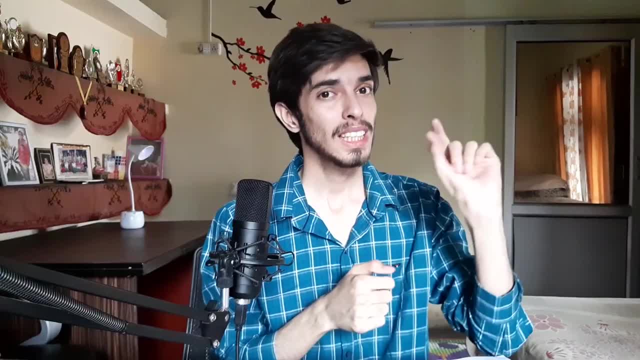 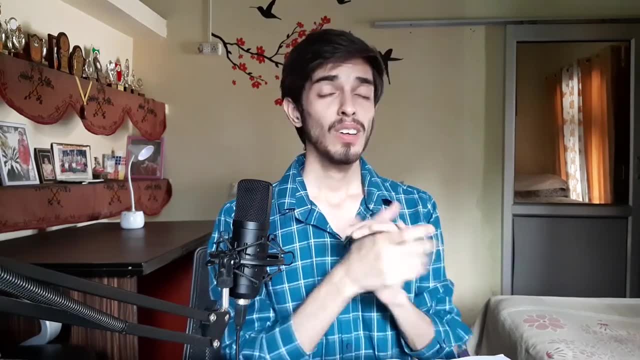 7 tends to 70. we have a remainder of 6. now 6 is the year code of 2061. now remember, in this one you don't need to consider that leap year exception. now let us see this trick in action. so let us see this trick in action. 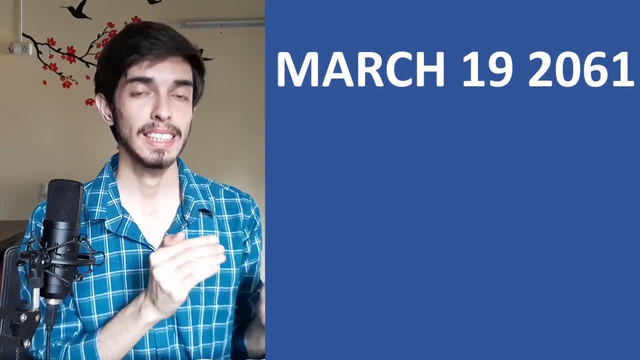 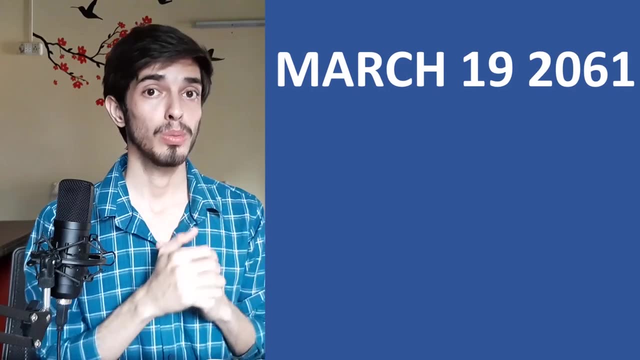 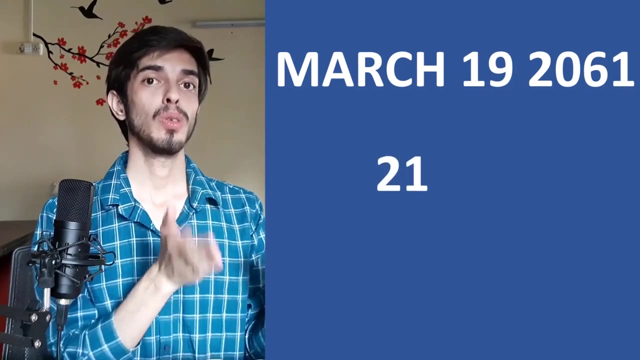 calculate the day of the week of march: 19, 2061. now what you need is really simple. see, we know the month code, we have memorized it. the month code of march is 2, the date is 19. add this 2, which is 21. now add the year code in this. like we have 2061. we have calculated this, which is 6. so 21 plus 6 is 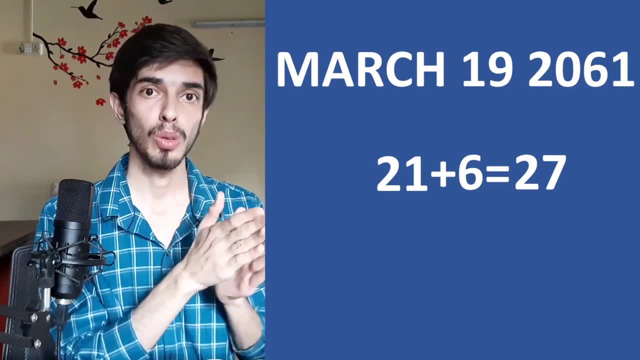 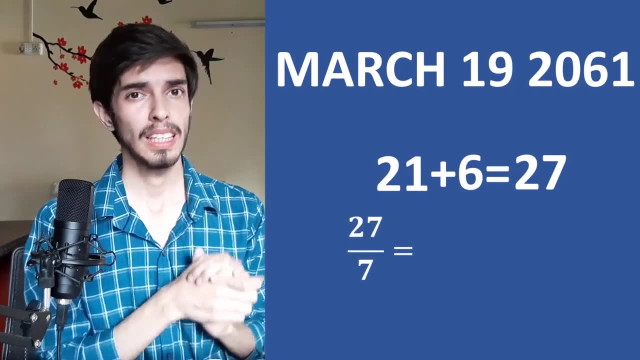 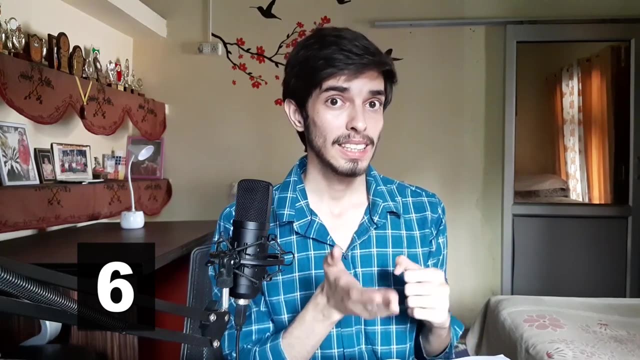 27. so basically you need to add all these codes together, all three codes. okay, so now basically divide this by seven. so see, division by seven is really important. so seventh is at 21 and the remainder is six. now this is our day of the week, so six is associated with saturday. so on march 19, 2061. 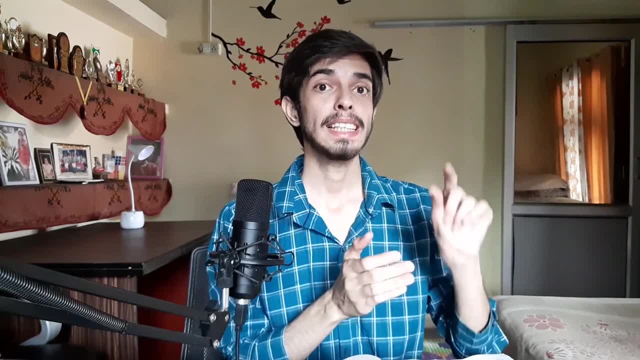 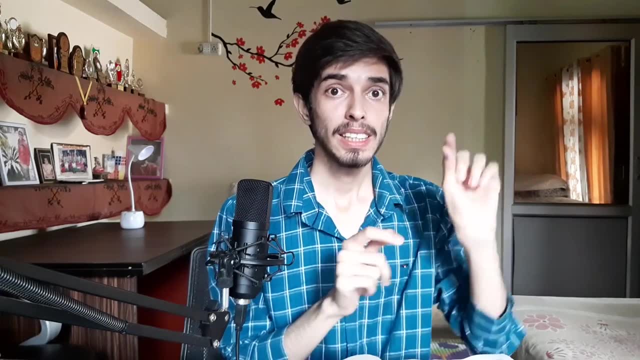 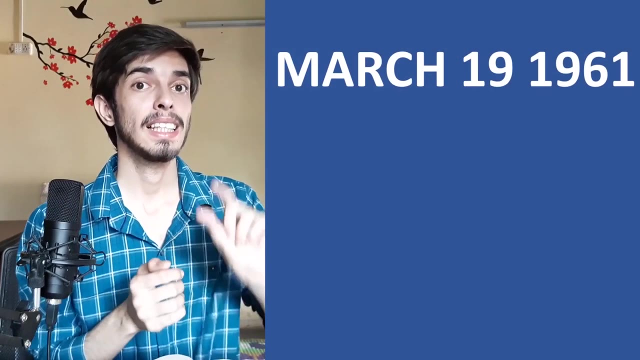 there will be a saturday. now what about the dates between 1900 and 1999? it is really simple. do the problem exactly same. just add one to the year code and you will get your code answer. So let's take an example: March 19, 1961. The same thing, but 1961 this time. So basically, 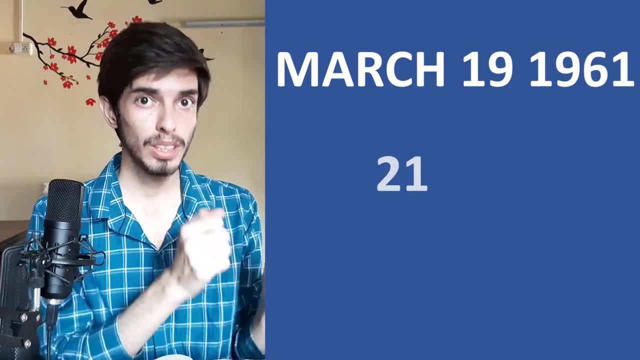 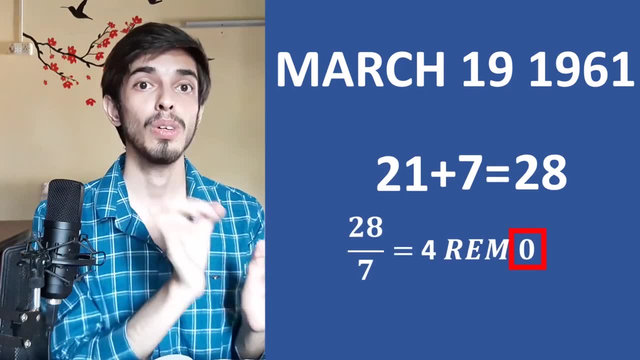 our year code would be 6, but now we need to add 1 to it, so it would be 7.. So our total would be 28.. So Sanfosa 28, so we have a remainder of 0, and 0 is associated with Sunday, So it was a Sunday on. 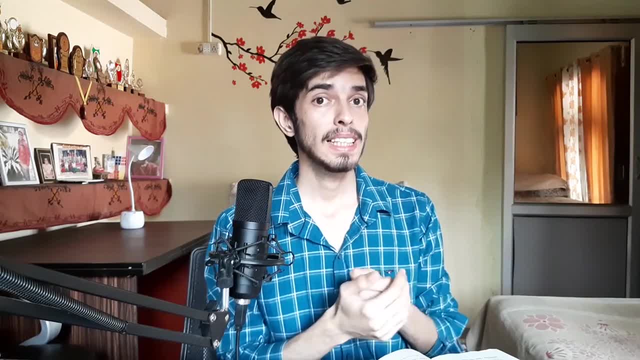 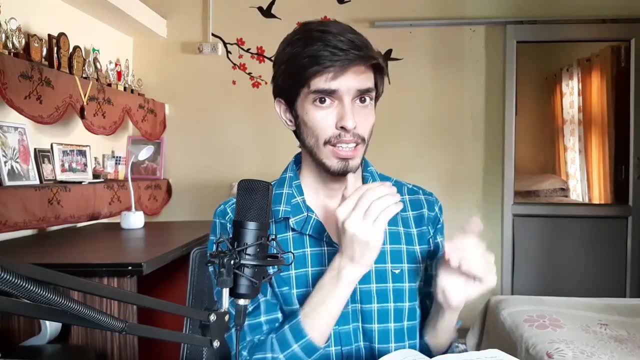 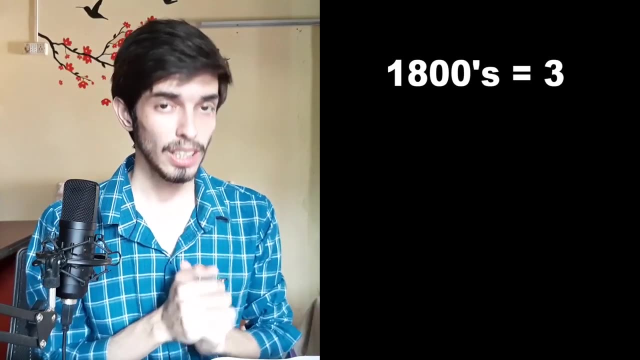 March 19, 1961.. Now for the dates in 1800s, we add 3 to the year code. and for the dates in 2100s, we add 5 to the year code. Now what I have told you this: for 1800s, we add 3 to the year code. 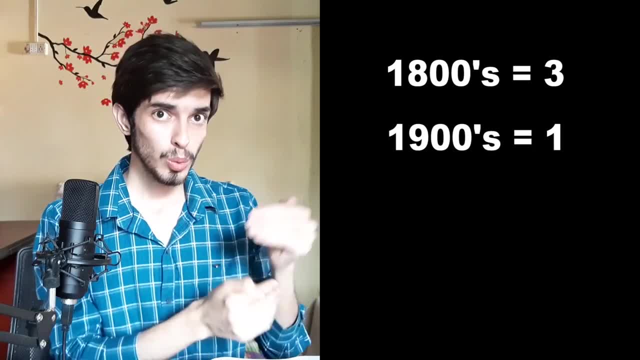 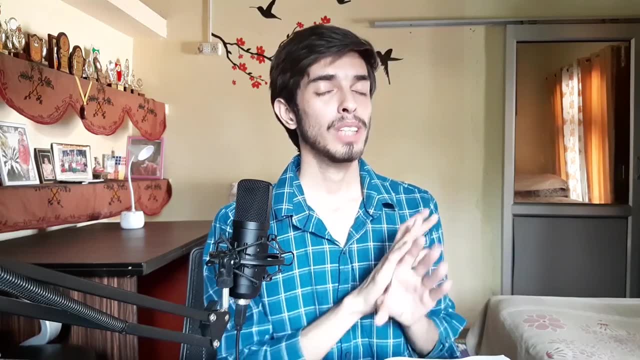 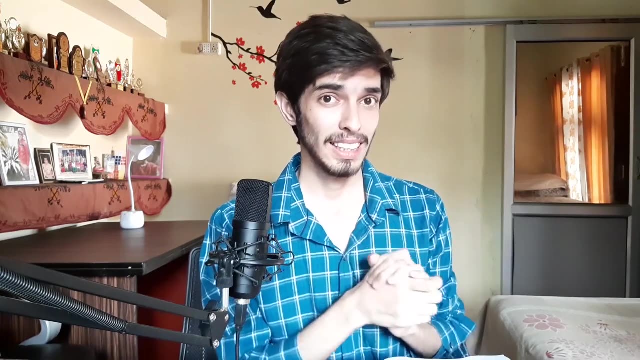 For 1900s, we add 1 to the year code. For 2000, we don't do anything. and for 2100, we add 5 to the year code. Now we have the power to calculate the day of the week of any date for these four centuries. Okay, now, the most interesting thing in here is that. 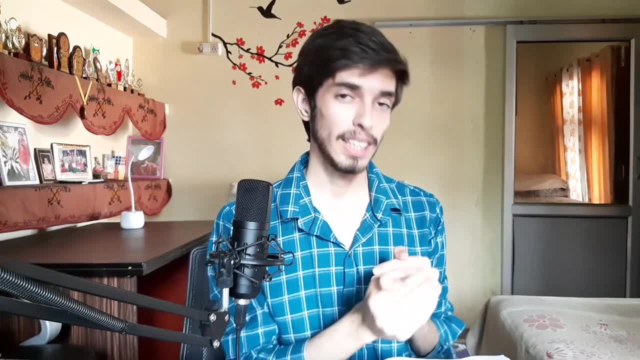 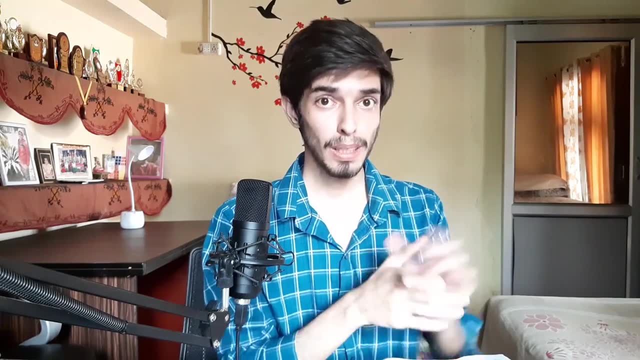 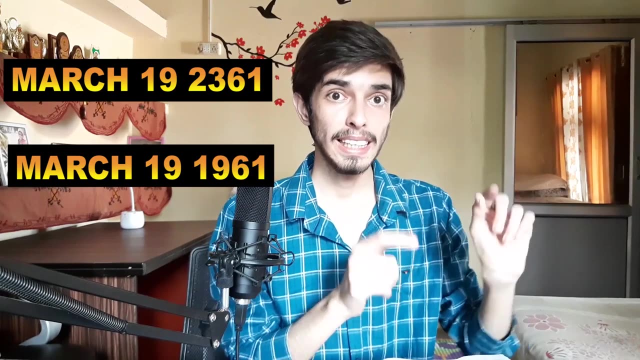 the Gregorian calendar repeats every 400 years. Okay, so if you can calculate for these four, you can calculate for any date. So see, it's really simple. March 19, 2361 would have the same day as March 19, 1961, because there is a 400 year gap between them. 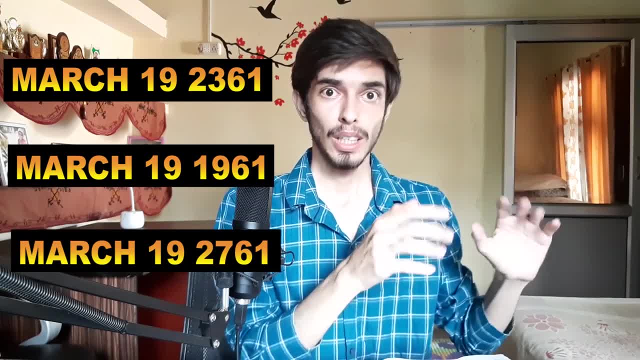 Similar to March 19, 2100,. there is a 400 year gap between them. similar to March 19, 2100.. So with this you can convert any date to a date near 2000.. For that you can calculate. 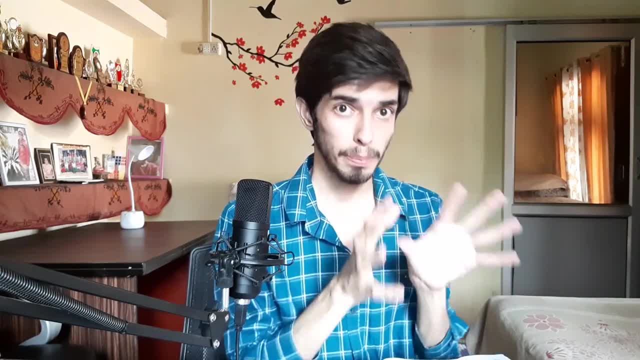 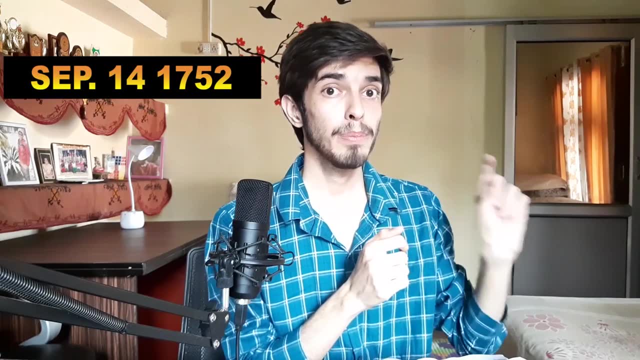 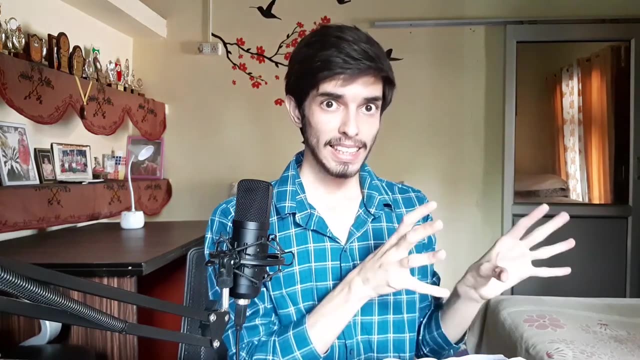 and this is only due to the fact that the Gregorian calendar repeats after every 400 years. So now I have a question for you: Calculate the day of the week of September 14, 1752.. So it was a Thursday on that day And at this day the Gregorian calendar was adopted. So if you go,